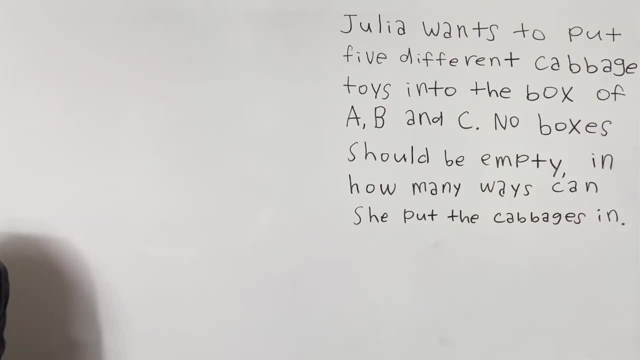 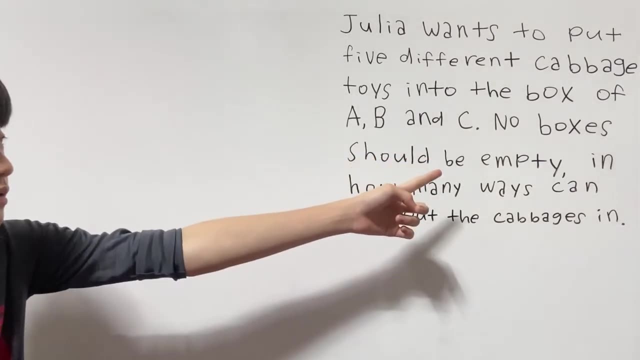 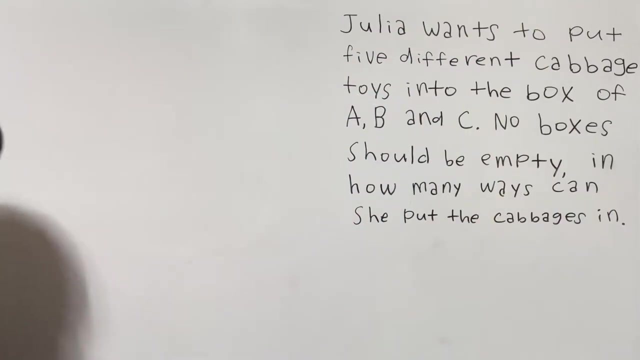 Hello everyone, and today we have a problem that Julia wants to put five different cabbages- cabbage toys- into the box of A, B and C. No boxes should be empty. In how many ways can she put the cabbages in? So to start off with this, 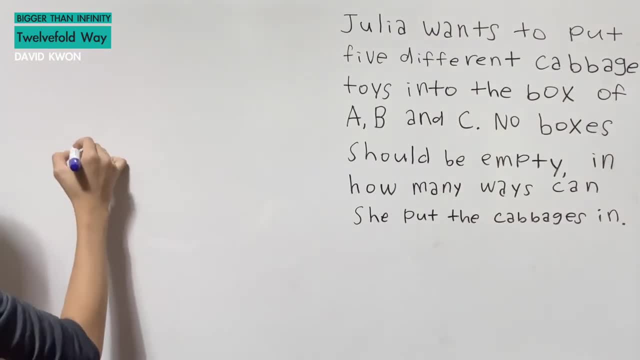 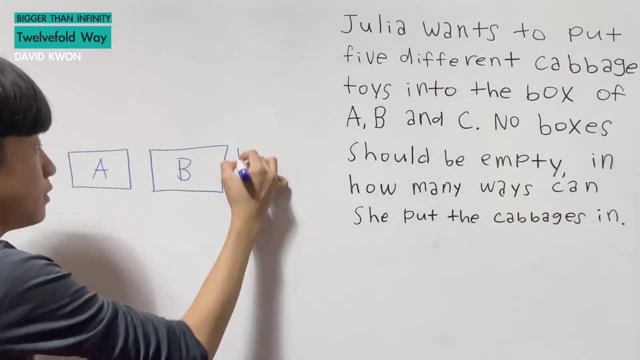 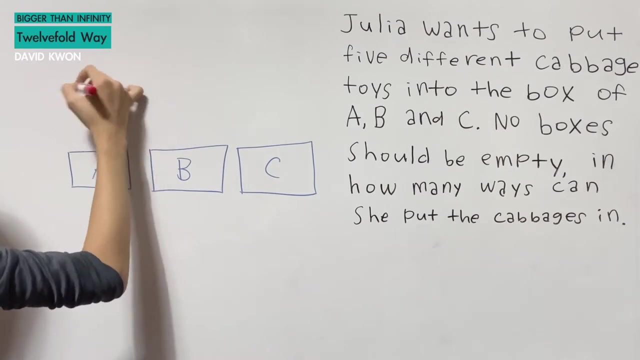 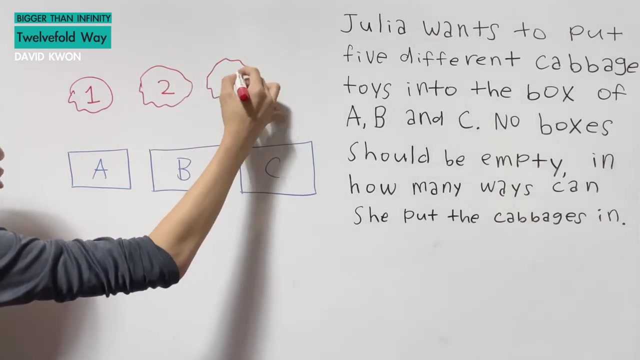 problem. let's draw. We have the boxes A and B and C. We also have five different cabbages and let's call that one, Cabbage number one, cabbage number two, cabbage number three, cabbage number four and cabbage number. 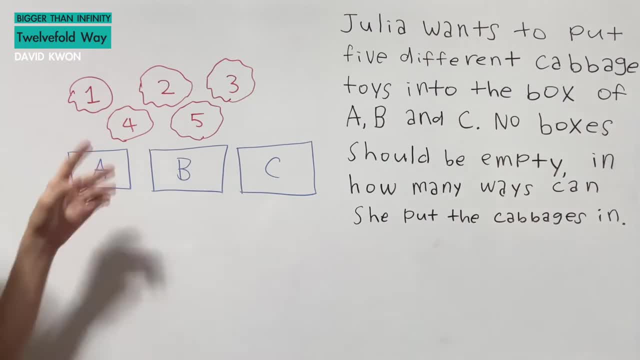 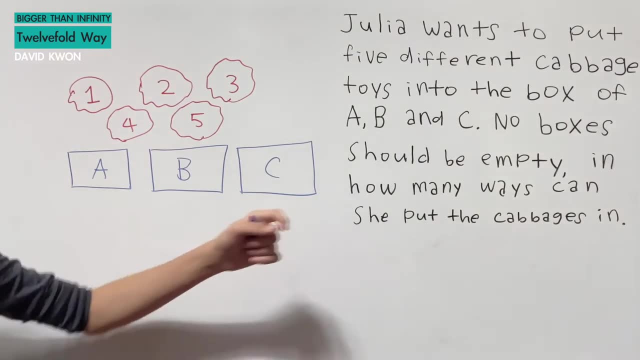 five. We want them to be inside the boxes and no boxes should be empty, So everyone has something to carry. So when it says no boxes should be empty, we do the opposite, which is from every boxes minus the opposite of no boxes. then we 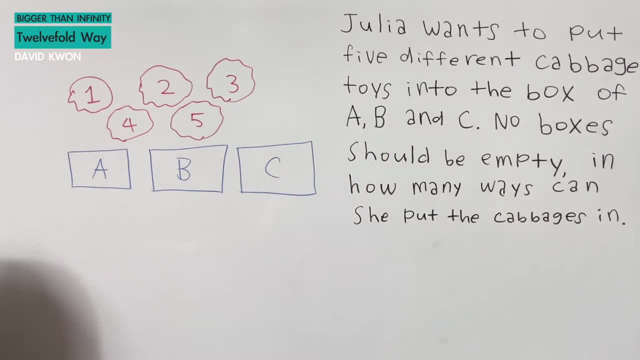 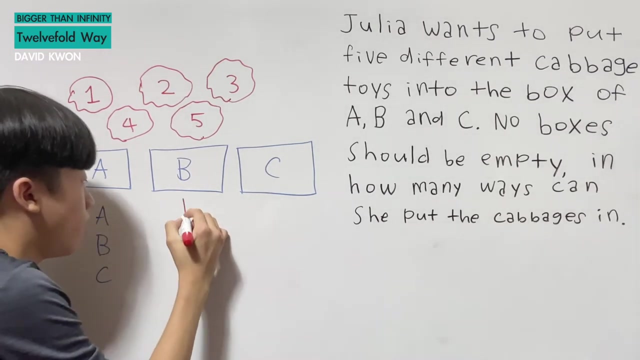 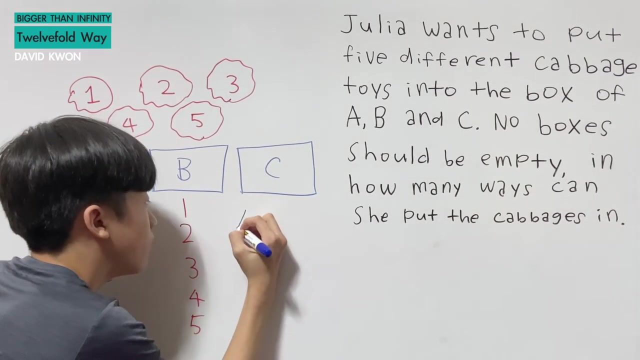 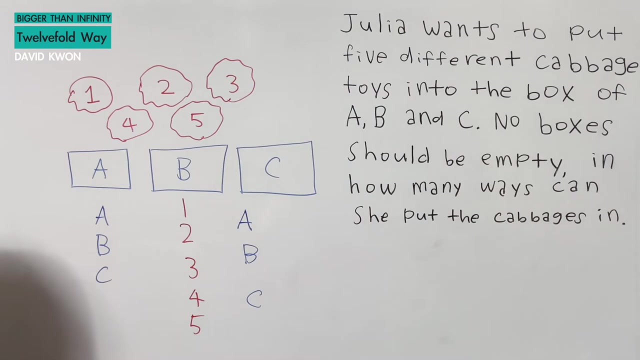 get. no boxes should be empty. So what did I just say? That is where I have all of them. All of them is the A, B, C, and we have one, two, three, four, five. I wrote it opposite. Okay, so no boxes should be empty. We don't care about that for now. 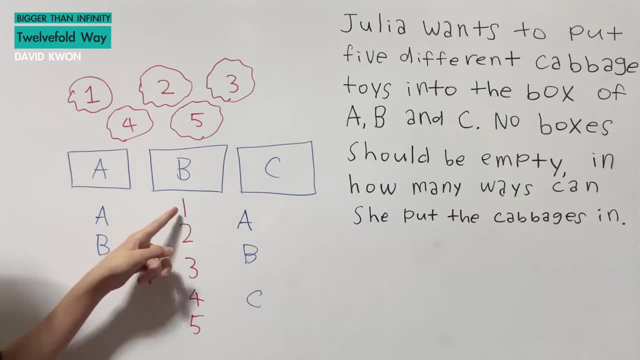 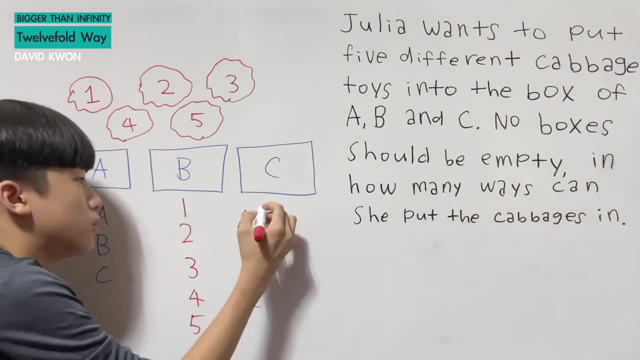 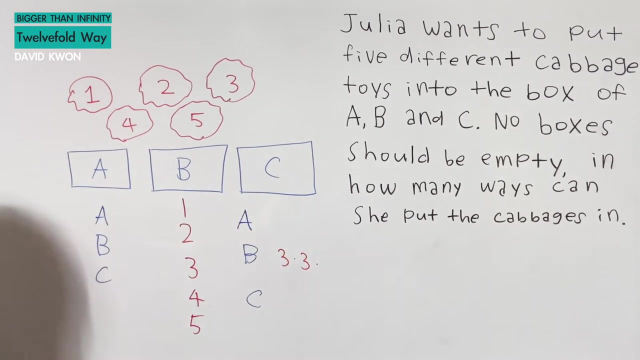 We want the word all Okay. so where can the cabbage number one go Go to? We have A, B, C boxes. Number one can go in three ways. Number two can go in three ways: A, B, C. Number three can go in three ways. Number four can go in three ways. I can go three ways. 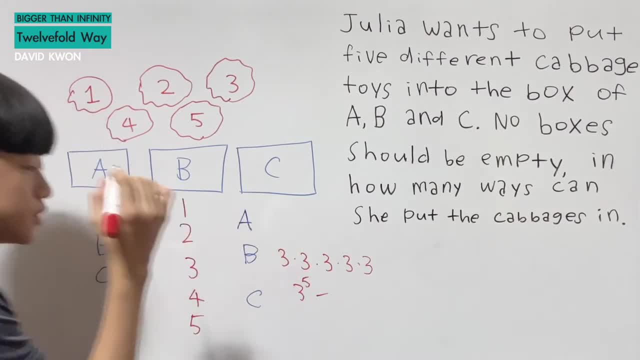 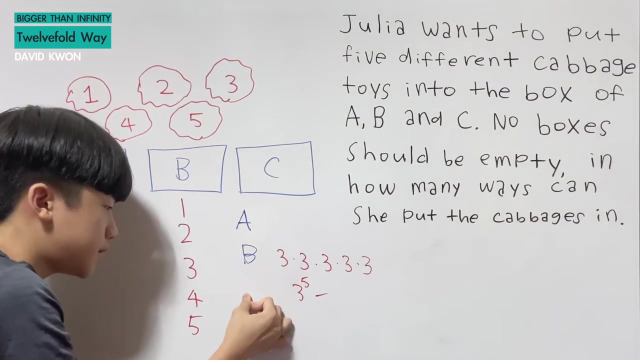 Just basically through to the power of five And let's subtract that by the opposite of no boxes. So basically let's count that we have no C, So we have one, two, three, four, five going to the box A and B.